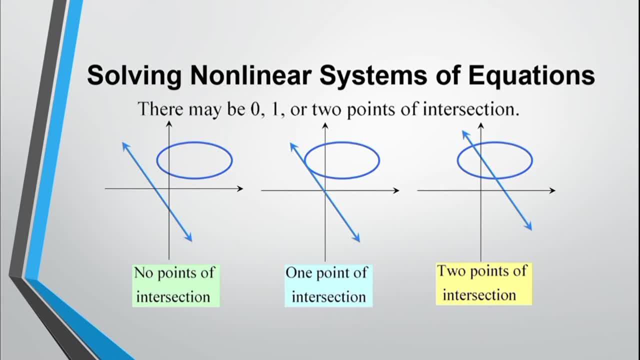 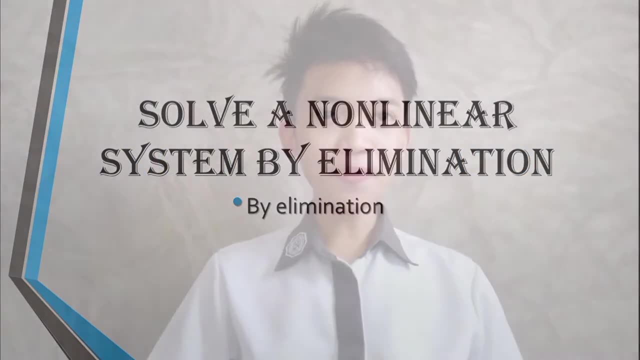 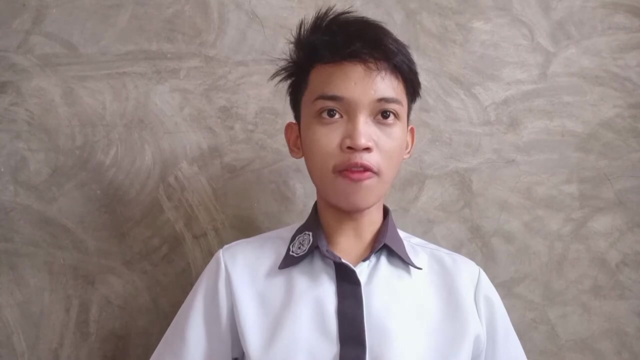 two points of intersection. So this is an example of the graph. So there are maybe zero or one or two points of intersections in solving nonlinear systems. In the elimination method you either add or subtract the equations to get an equation in one variable When the coefficients of one variable are. 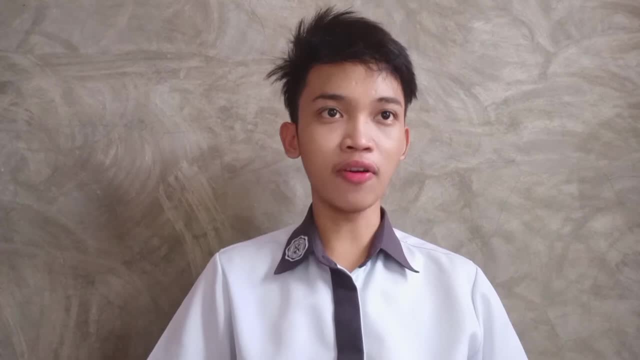 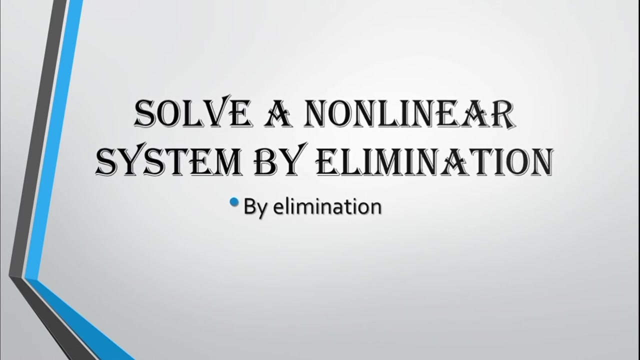 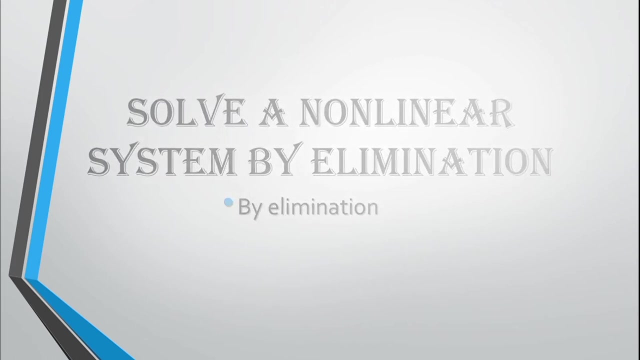 opposites, you add equations to eliminate a variable, and when the coefficients of one variable are equal, you subtract the equations to eliminate a variable. We can also use elimination to solve systems of nonlinear equations. It works well when the equations have both variables squared. When using elimination, we tried to make the coefficients of one. 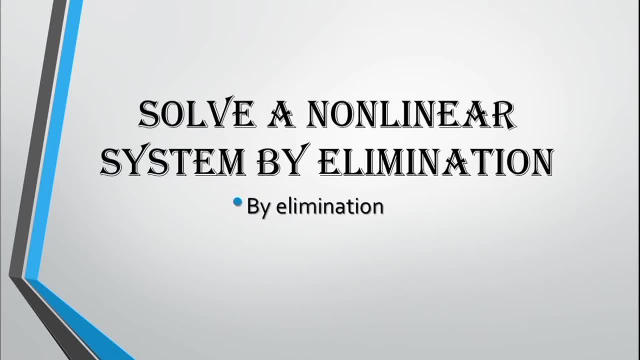 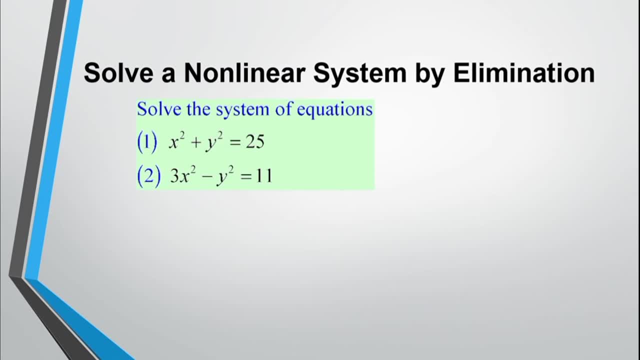 variable to be opposites. So when we add the equations together, the coefficients of that each of them are equal. So we were able to calculate the актив, το wav c par oneAT-mk. that variable is eliminated. So let's give an example on how to solve a nonlinear system by 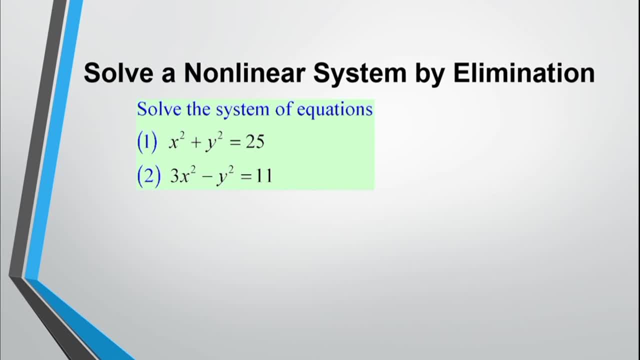 elimination. So number 1, x squared plus y squared is equal to 25.. Number 2, 3x squared minus y squared is equal to 11.. So the graph of equation is a circle and the graph of equation 2 is a. 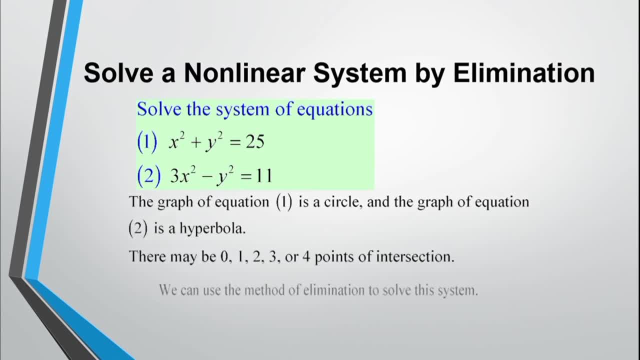 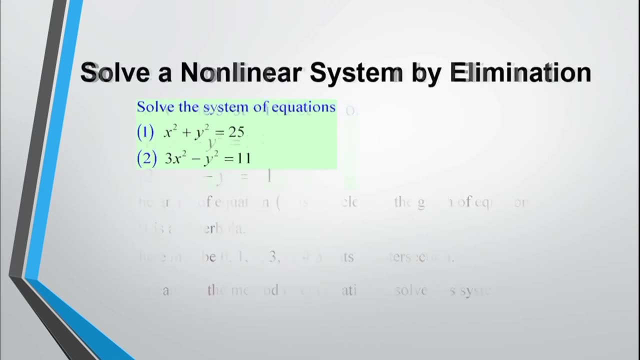 hyperbola, So there may be 0,, 1,, 2,, 3, or 4 points of intersection. We can use the method of elimination to solve this system. So the first one is circle and the second one is a hyperbola. So adding the 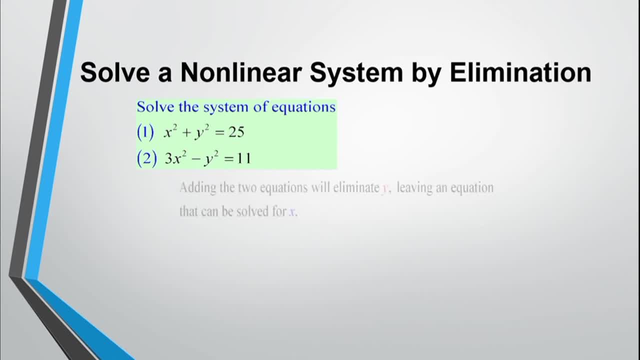 two equations will eliminate the y variable, leaving an equation that can be solved for x. So here's the solution: x squared plus y squared is equal to 25.. 3x squared minus y squared is equal to 11.. So the final solution is: 4x squared is equal to 36.. 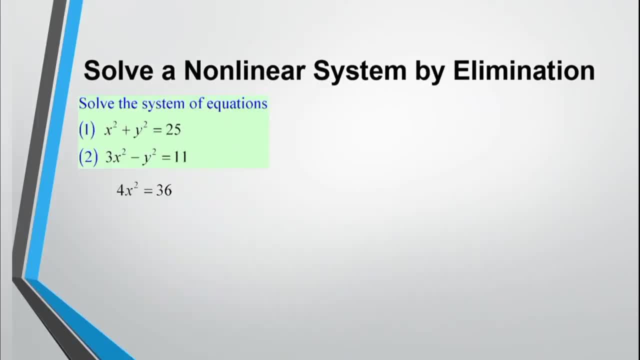 So our last final answer will be: 4x squared is equal to 36.. So we should divide both sides by 4, solve for x, So it should be x squared. x squared is equal to 9 and x is equal to positive negative 3.. So we should have: